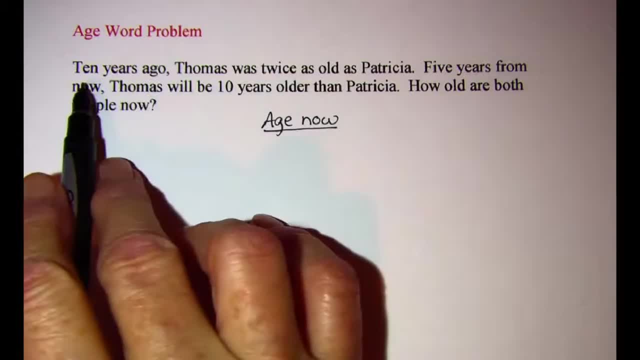 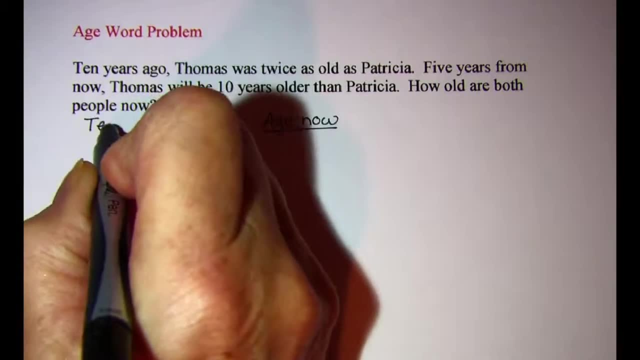 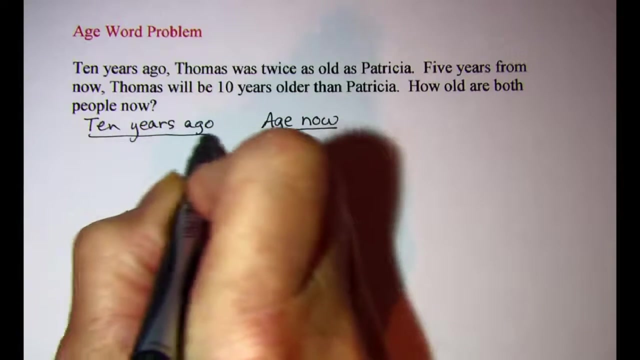 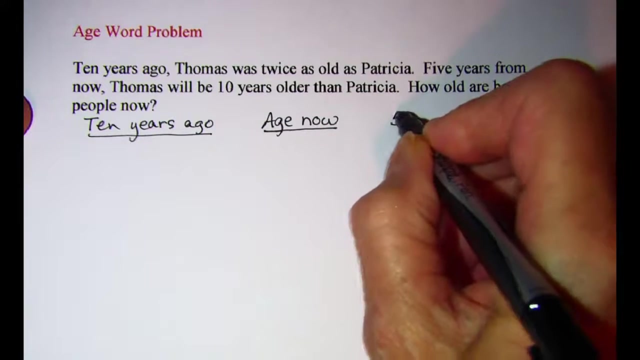 and you have that column And then I have ten years ago, So I'm going to set up a column that's labeled ten years ago, And then I also have five years from now, So I'll set up a column that's labeled five years from now. 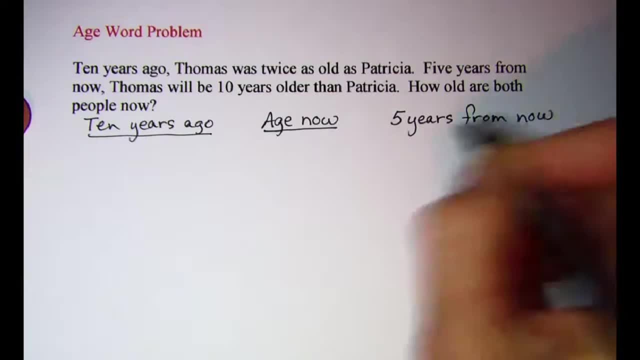 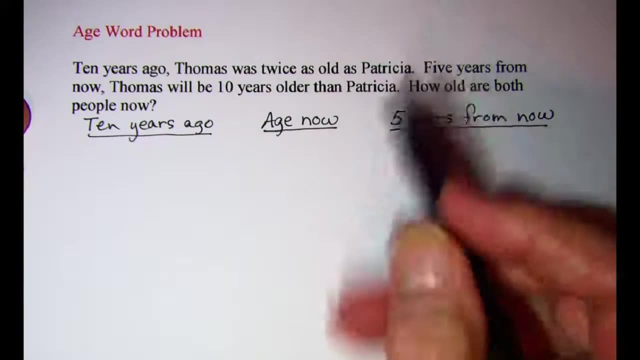 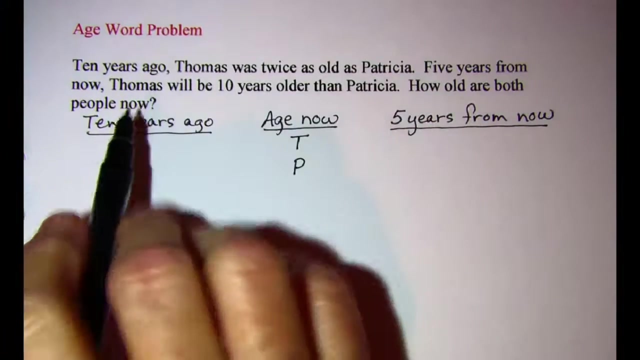 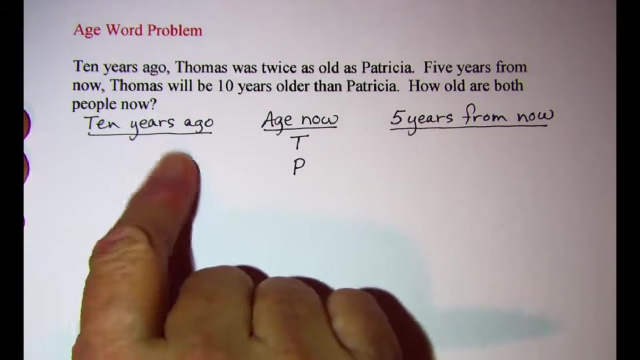 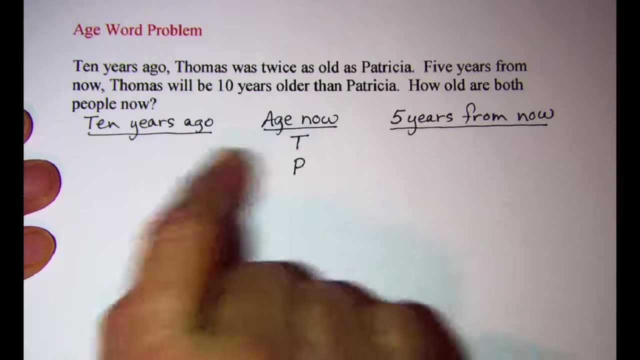 Now I'm going to use t and p as the variables. My first sentence talks about ten years ago, So I'm going to fill in my variables for ten years ago. If Thomas is t years old, how old is he? If Thomas is t years old now, ten years ago he would have been t minus ten. 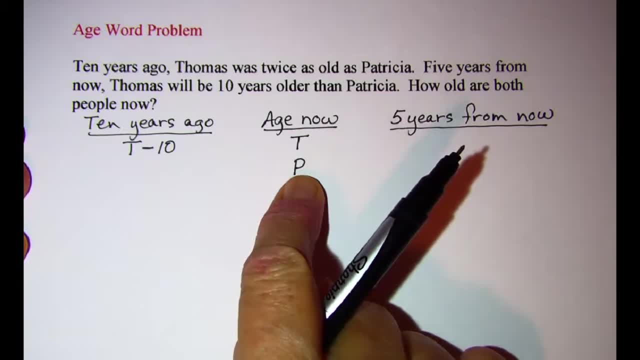 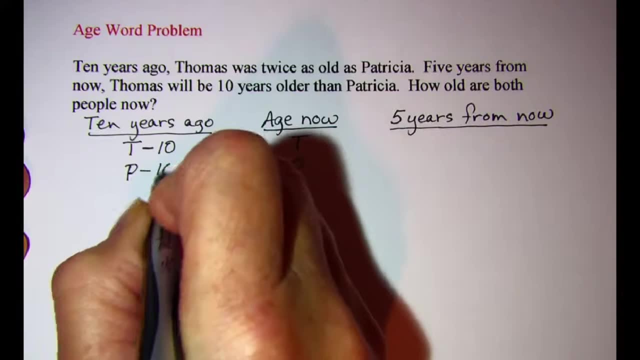 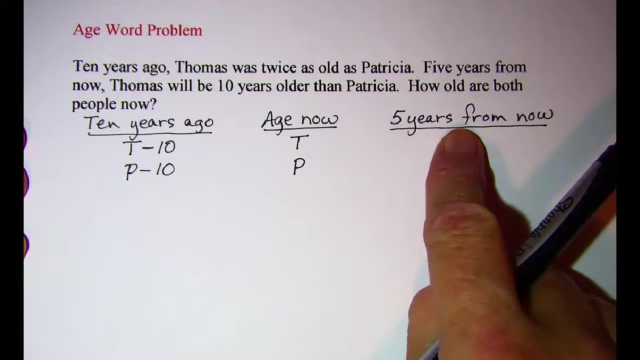 And p is Patricia's age now. So ten years ago Patricia would have been p minus ten. Now let me also fill in their ages five years from now. Thomas is t Now, so five years from now he will be t plus five. 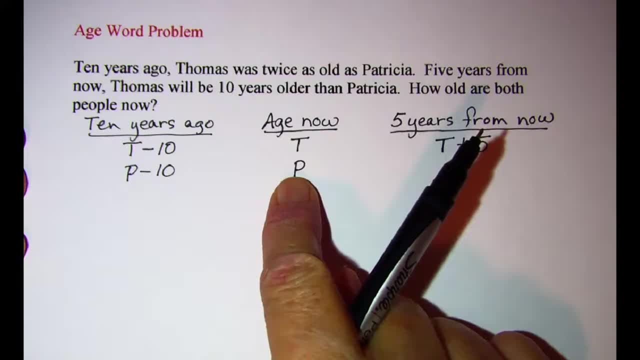 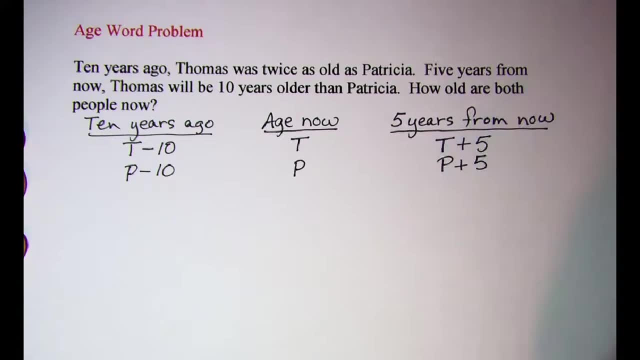 And p is Patricia's age now. So five years from now she will be p plus five. So now I have the variables ready to translate these two sentences. So now I have the variables ready to translate these two sentences, This first sentence. we're talking ten years ago. 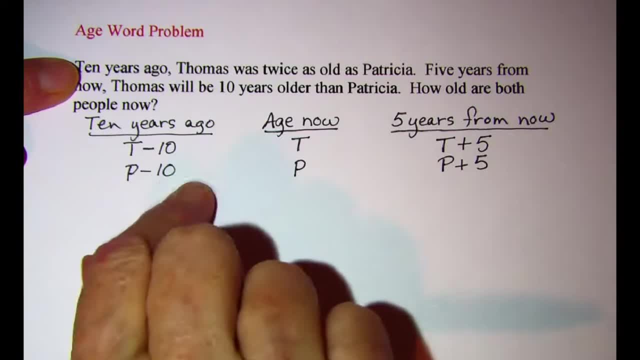 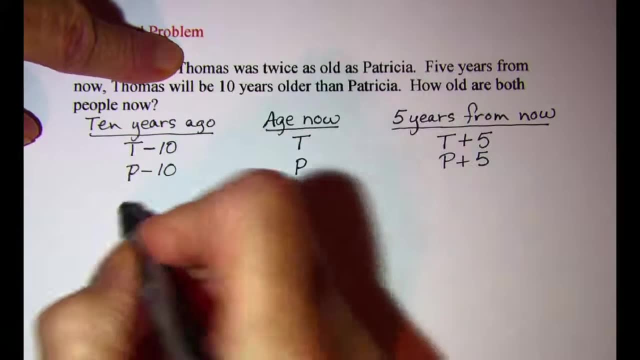 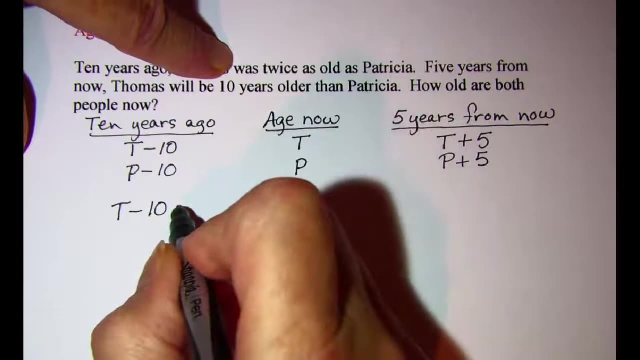 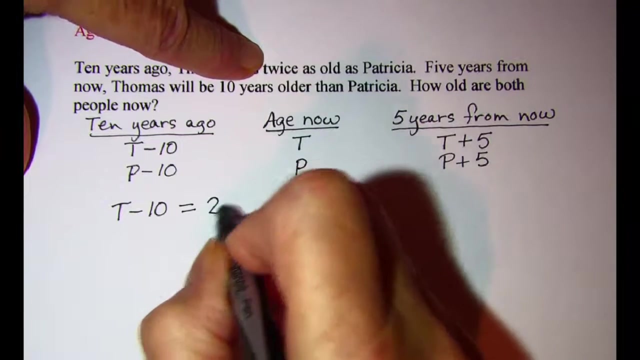 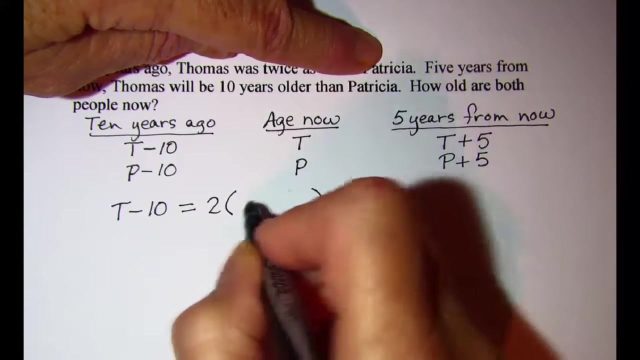 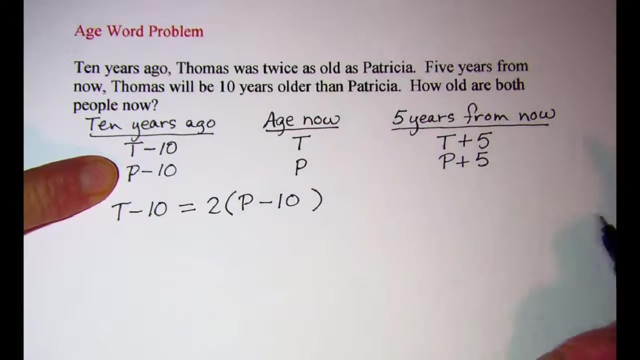 so I'll just be using these expressions. when it says Thomas and Patricia, So Thomas, I'll write t minus ten Was, that's our verb, so that's where the equals goes. twice, that means two times as old as Patricia. So in the parentheses here I'm going to put Patricia's age 10 years ago, so p minus 10.. 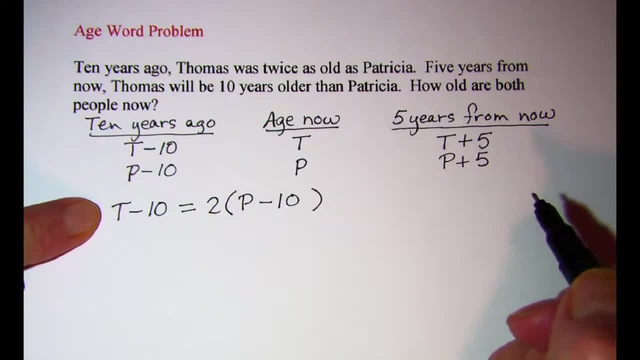 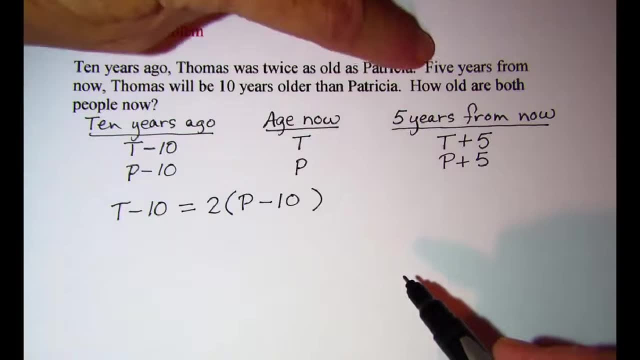 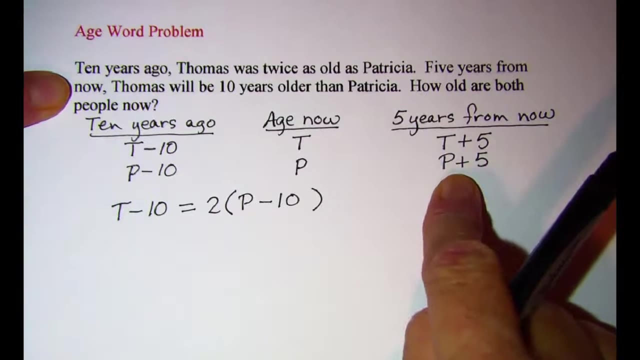 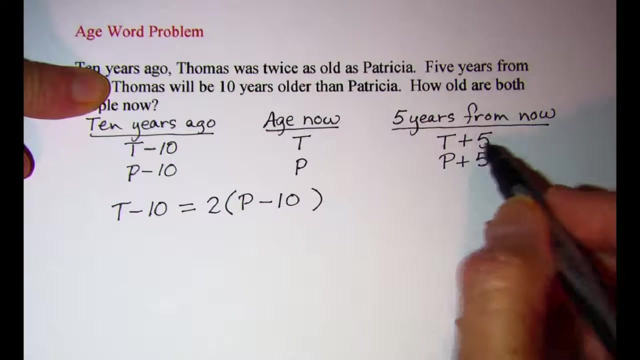 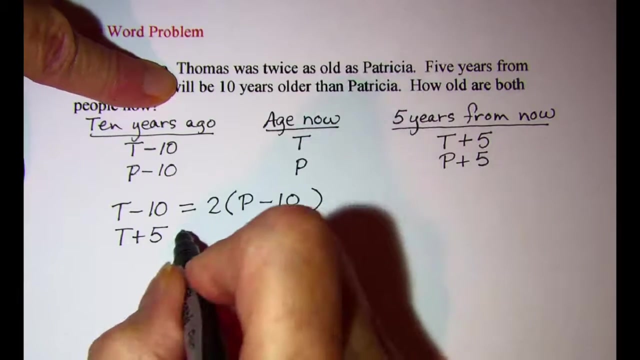 So this is my first equation that I'll be working with. Now. let's use the second sentence to translate: It starts with five years from now, so I'll be using these expressions whenever I see Thomas or Patricia Thomas, so t plus five will be- and that's our verb- where the equals goes 10 years older. 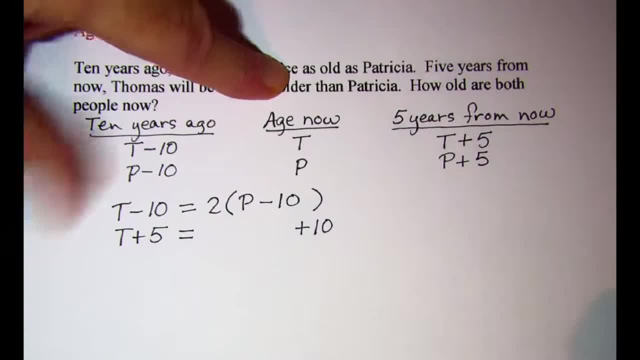 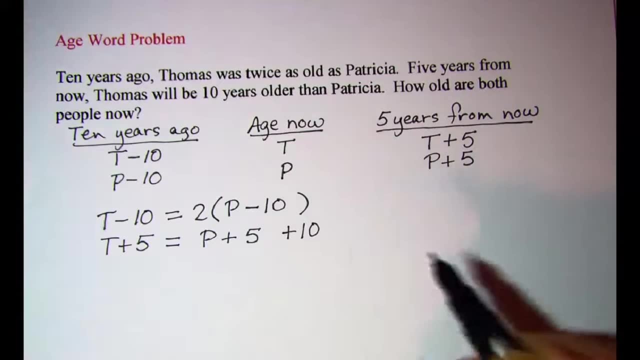 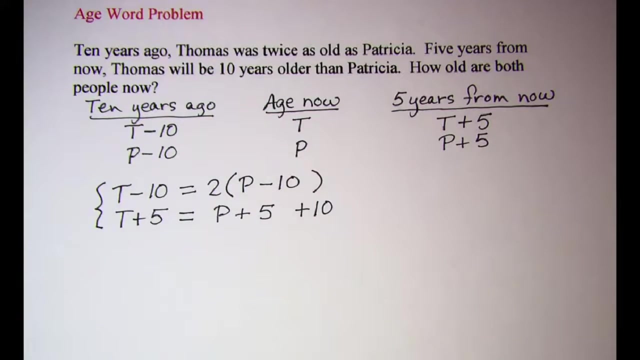 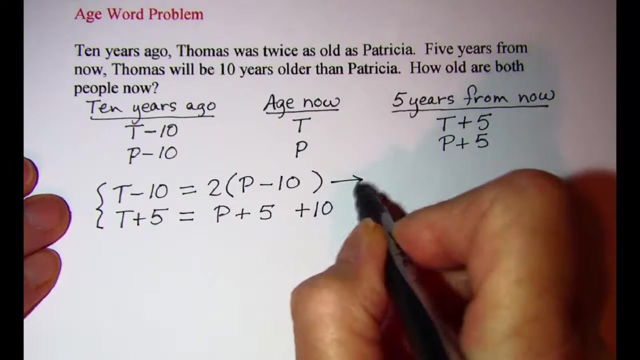 So I'm going to be adding 10.. 10 to something, Then Patricia, So p plus five. So these are my two equations that I need to solve now. On this one, I'm going to distribute my two first, So I have p minus 10,. 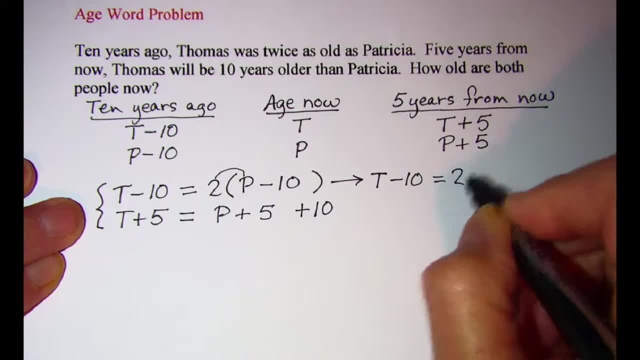 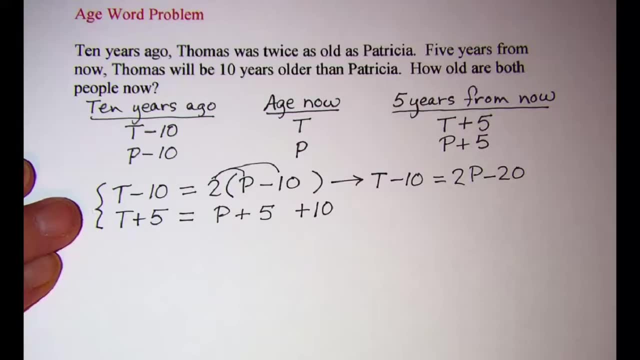 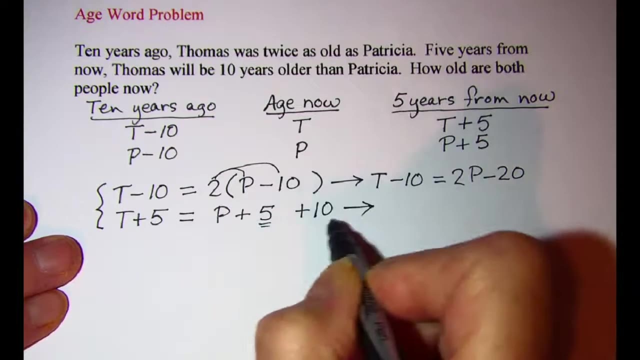 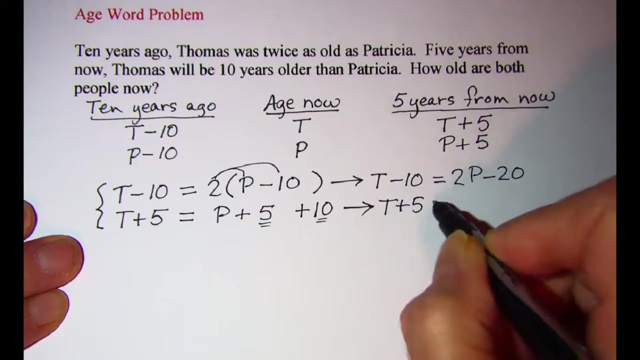 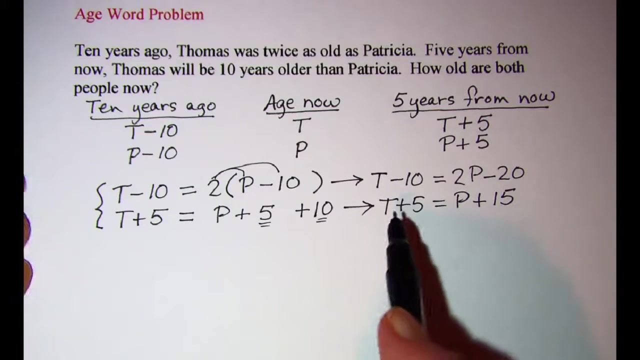 equals two p minus 20.. And then on this one, I'm going to combine my constants over here: t plus five equals p plus 15.. My next step: I'm going to rearrange these two equations so they kind of look alike. 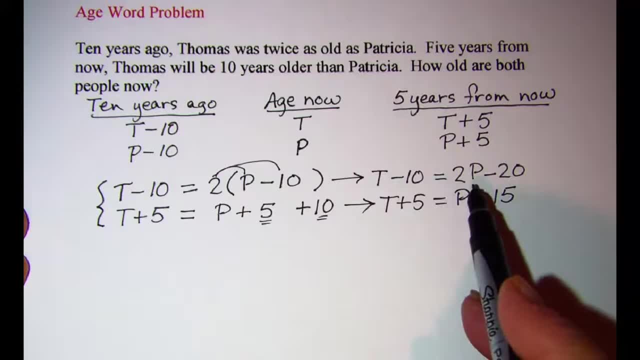 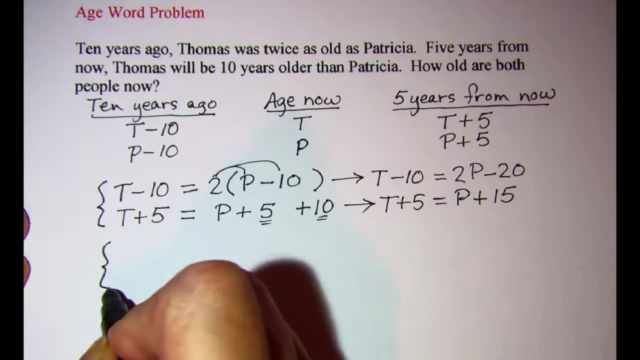 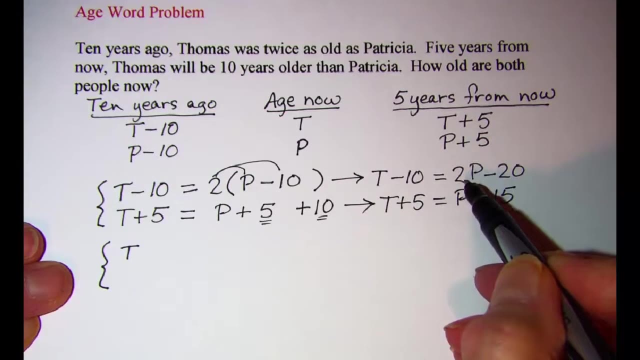 And usually I'll put both of my variables on the left and my constants on the right and then see what method I want to use to solve. So my t is already on the left. I'll move my two p to the left. 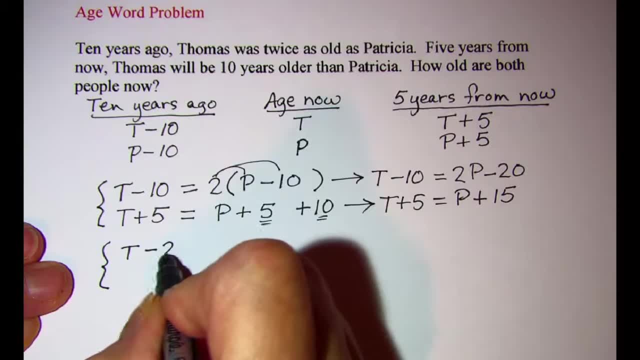 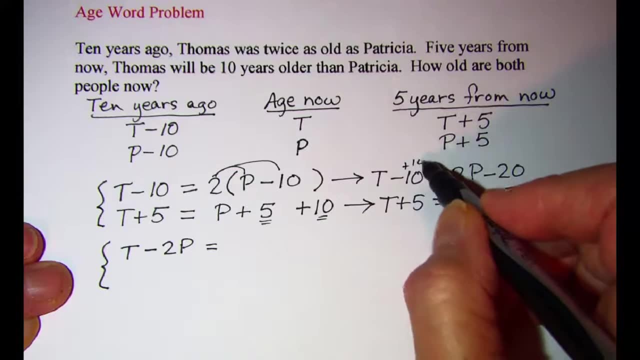 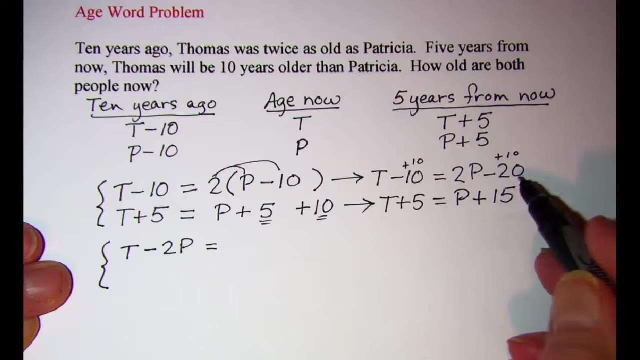 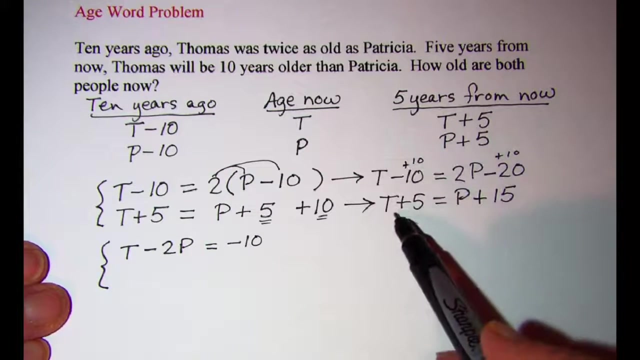 by subtracting two p from both sides And then I'll add 10 to both sides to move my numbers to the right. So 10 and negative 20, is negative 10.. For this equation my t is already on the left. 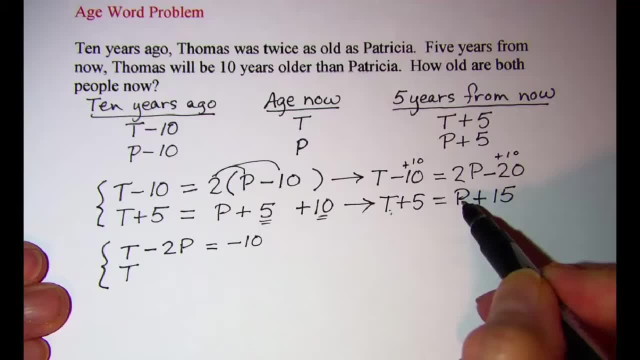 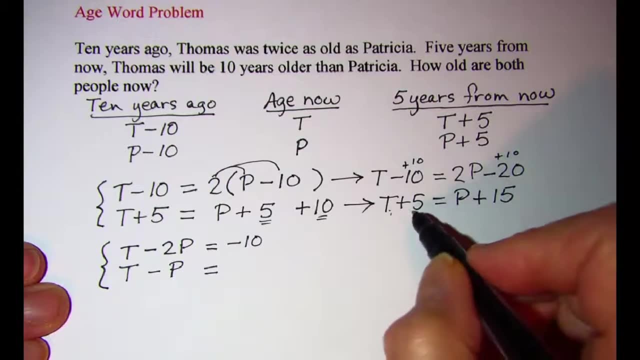 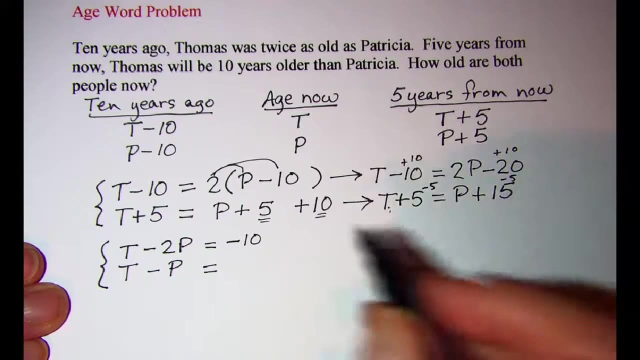 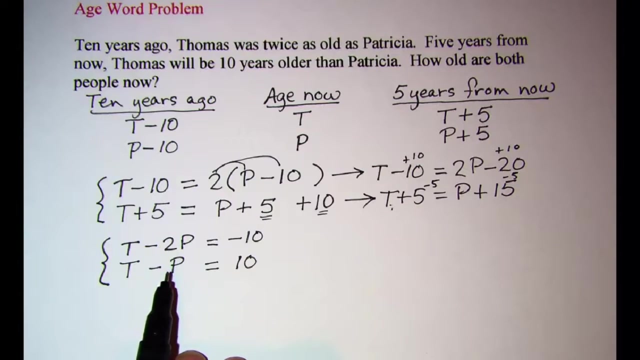 So I'll just copy it: Subtract p from both sides to move my p to the left, And then subtract 5 from both sides, So I have a 15, subtract 5 is a positive 10.. Now you can choose what method to solve this system. 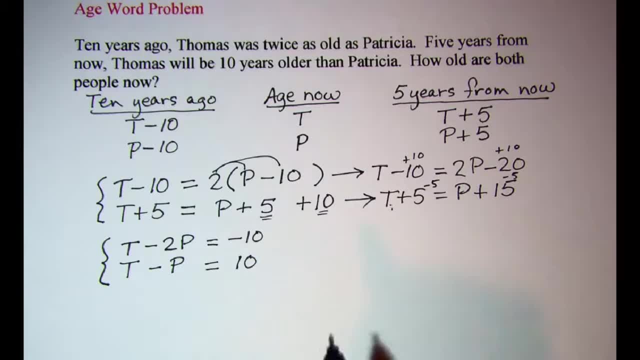 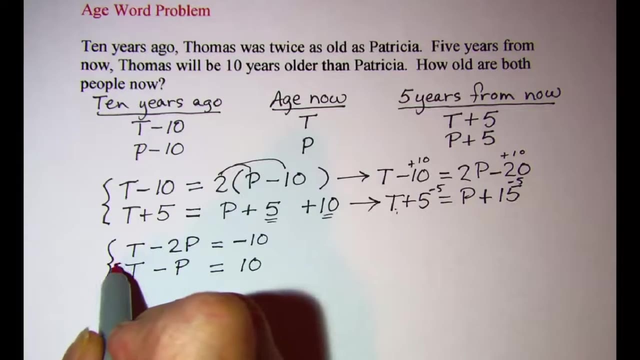 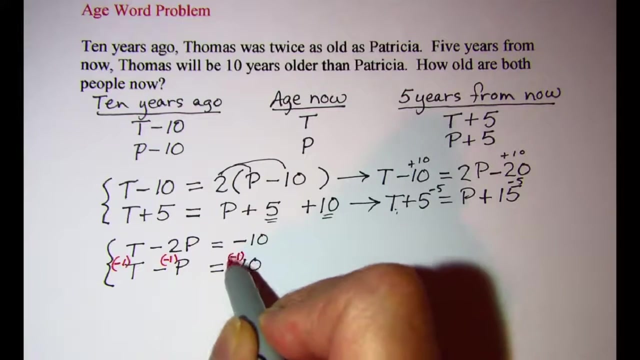 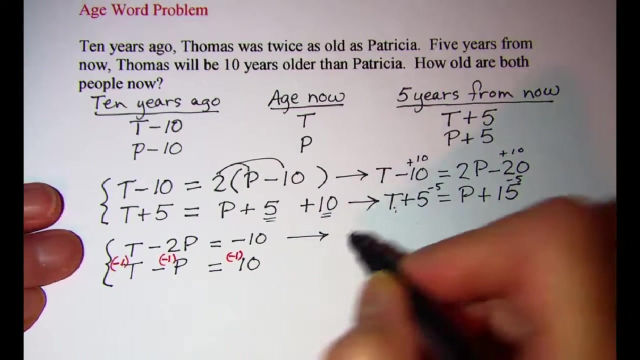 Either elimination or substitution. My preference is elimination, So I'm going to multiply every term on this second equation by a negative 1.. And then we copy these. So this one- I haven't done anything to that- I have t minus 2p. 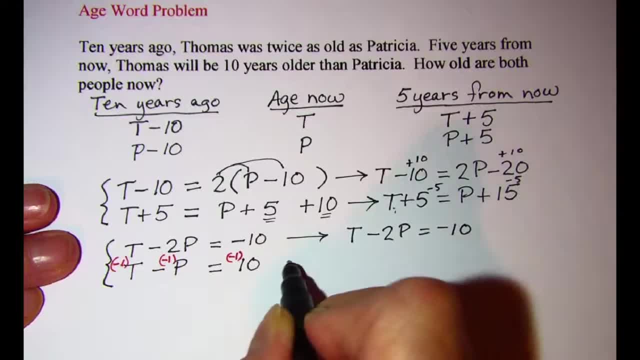 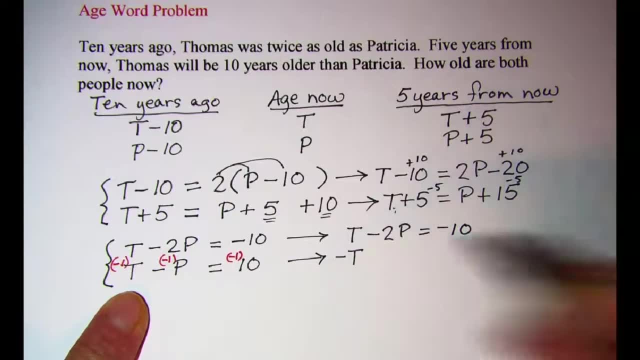 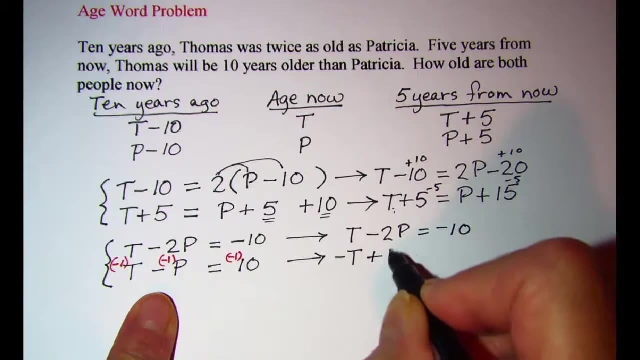 equals negative 10.. This one, now a negative 1 times t, will give me a negative t. A negative 1 times a negative p will be a positive p And then a negative 1 times 10, is a negative 10.. 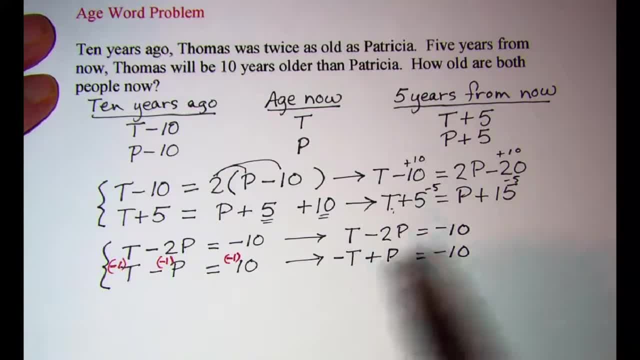 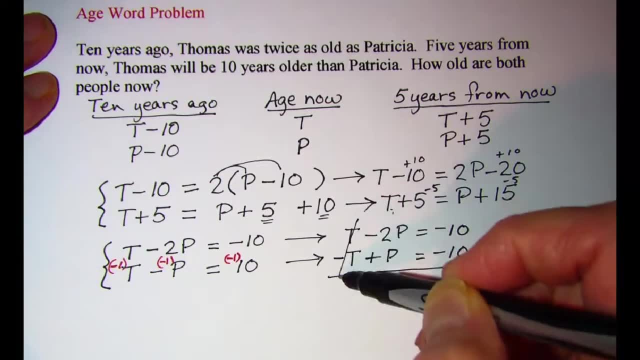 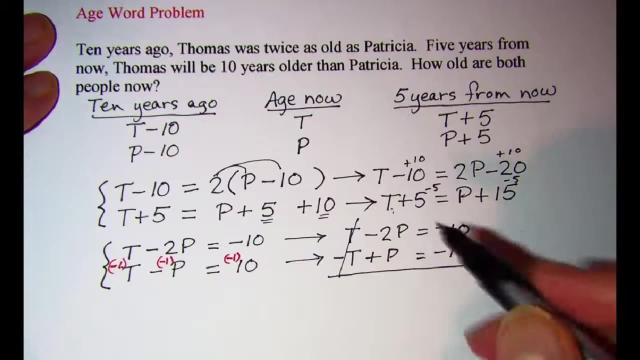 Now these two equations are ready to be added together so that I can eliminate the t's. Whenever you have a positive and a negative same variable, those go away. So negative 2p and a positive 1p is negative 1p. 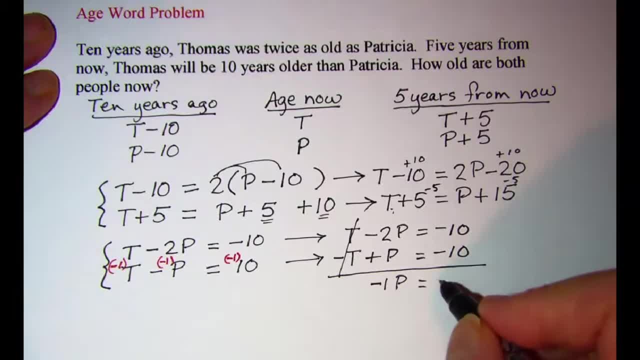 Negative 10 and negative 10, is negative 20.. I'm going to divide both sides by negative 1. And p is equal to 20.. So this is Patricia's age, which is 20 years old. Now, once you have one of the answers,